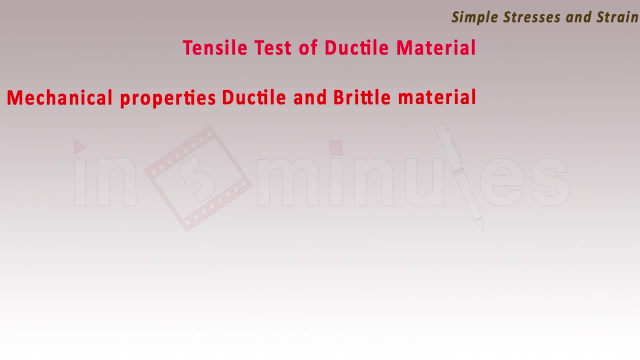 properties of most of the materials, whether ductile or brittle, can be easily studied by a test called as tensile test. Now, tensile test. what is tensile test? Tensile test can be carried out on a standard specimen of the shape as shown in the figure diameter. 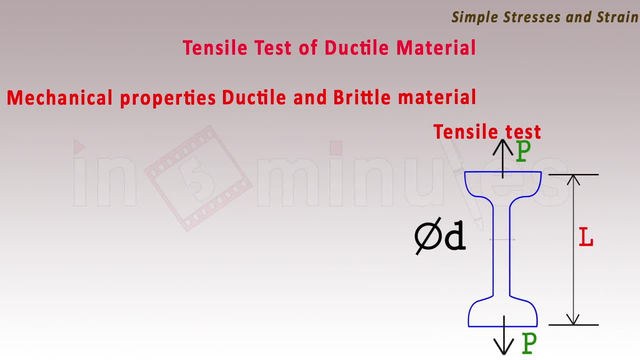 D and length L by applying tensile load on its axis. Tensile load is carried out on a machine called universal testing machine. The specimen is loaded between the two jaws of the machine and by hydraulic means loads are applied so that tensile load is applied. 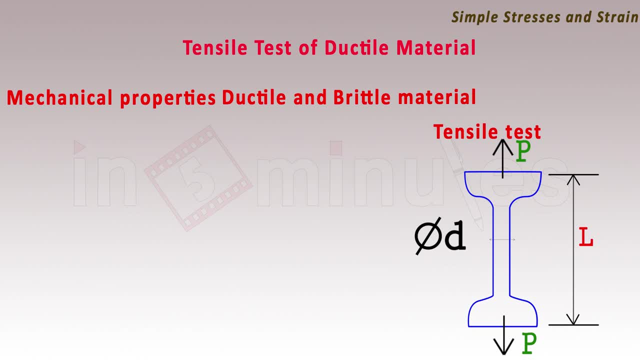 on the specimen As the loads are applied. we can measure the 2 properties of tensile test In the tensile test as the load is applied and gradually increased. we can continue continuously measure properties, which is sigma is given by P upon A, where A is the original. 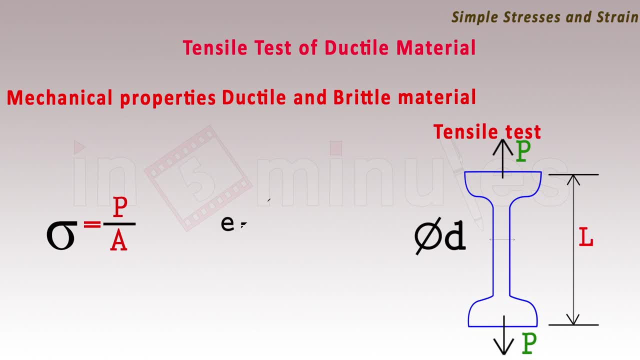 cross-sectional area. We can also measure the strain E, which is given as delta L by L. The tensile test is carried out on the specimen until the specimen fails or breaks. From the start of test up to the failure, we measure the stress and strain and we plot. 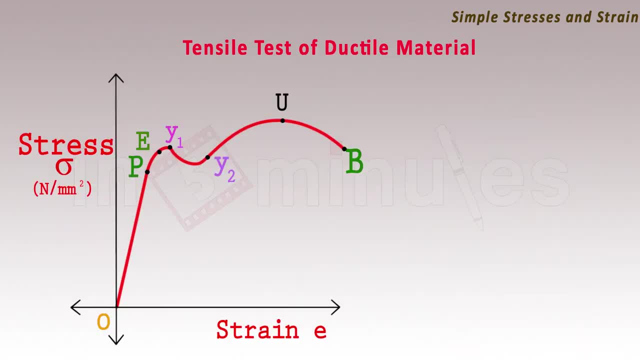 it on a diagram called as stress-strain diagram. We plot the stress on y-axis and strain on x-axis. This curve is a typical stress strain curve for any ductile material. Initially, when no load is applied, we have stress is equal to 0 and strain equal to 0.. It is denoted. 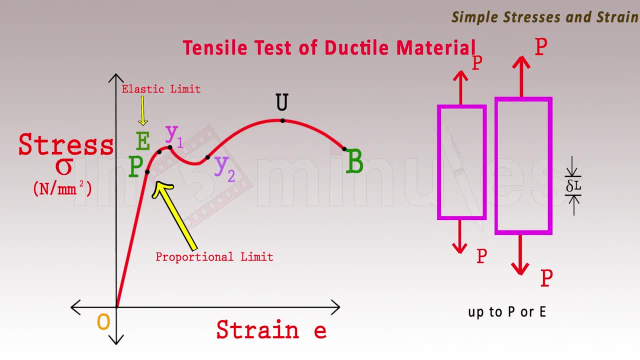 by point o. As the load is gradually increased, we see that the stresses are developed in the specimen and the specimen elongates, as shown in the figure delta L. So the stress-strain curve increases in this fashion As load is gradually increased, both stress and strain. 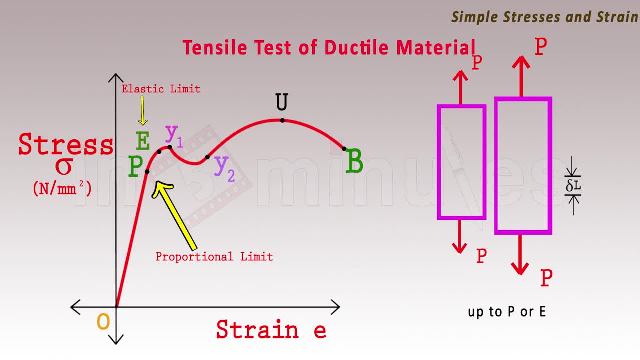 increases. It has beenじ found that the material elongates and the stress is directly proportional to strain upto some load, ie the ratio of stress and strain is constant. This fashion continues upto point P. the material is said to be in an elastic state. 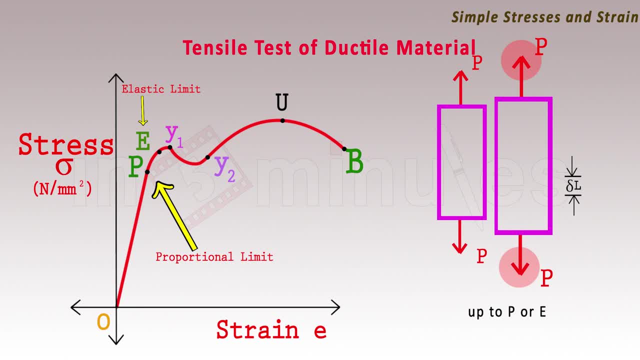 Elastic state means that when the applied load is removed, the material again go back to its original size and shape. As the load is gradually increased, we see that both stress and strain increases and the material elongates. as shown in the figure From point O, the stress is directly proportional to strain and it has been found that the ratio 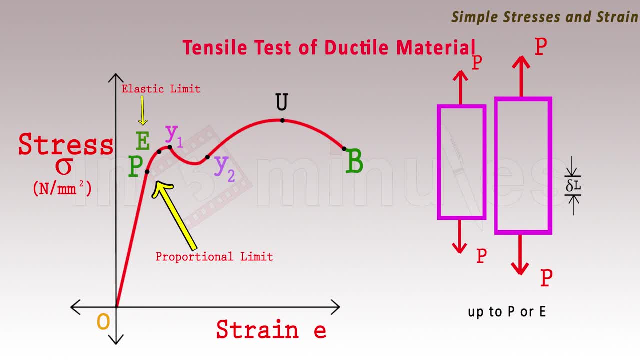 of stress and strain is constant. This fashion continues upto a point called as proportional limit. The material is said to be in an elastic state. Elastic state means that when the applied load is removed, the material again go back to its original size and shape. 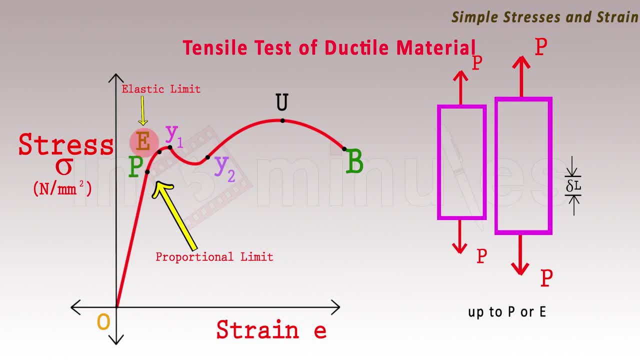 Now, beyond point P, there is a small region, upto point E, where the material still exists in elastic state, But the stress and strain is no more, So point E is called as elastic limit. Even if the load P is removed, the material won't go back to its original size and shape. 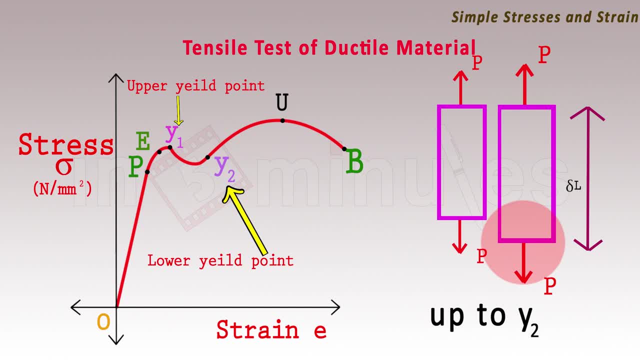 That means there will be permanent set of deformation induced in the bar or specimen. Now this plastic region is also called as yielding region. Yielding has a characteristic that there is a considerable increase in strain in this region and negligible increase in the stress. Now the curve follows an S path. 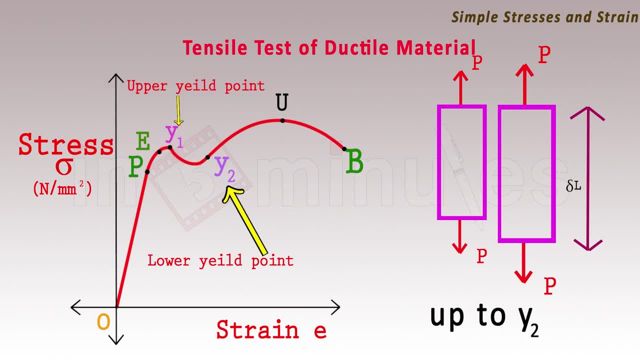 The point of maximum stress on this yielding region is called as upper yield point. There is a point of lowest stress In this yielding region is called as lower yield point. Upon further increasing the load beyond point Y2, there is a considerable increase in load. 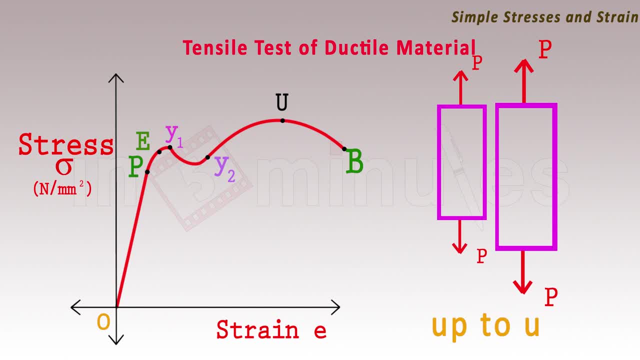 for further straining, And this is due to the phenomena called as strain hardening. This curve again rises up and point U is called as ultimate tensile point or ultimate tensile strength of a material. Ultimate tensile point is the maximum stress encountered in a tensile test of a material. 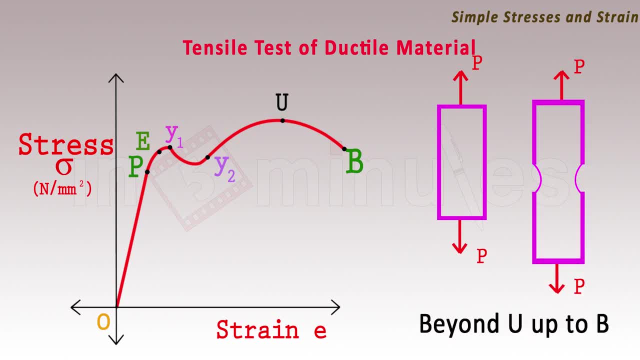 Beyond point U, We see that there is a localized reduction in the cross-sectional area at the weakest point of the material. This is called as necking. This continues until the material finally breaks. Now, due to the reduction in the cross-sectional area, the required load to further strain. 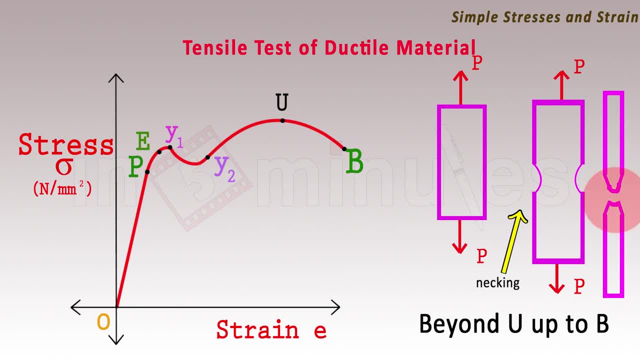 decreases and eventually the material breaks, That is, it breaks into two pieces. The failure which takes place for a ductile material is called as cup and cone failure, Meaning that one piece of the broken specimen has a cup shape And another has a cone shape. 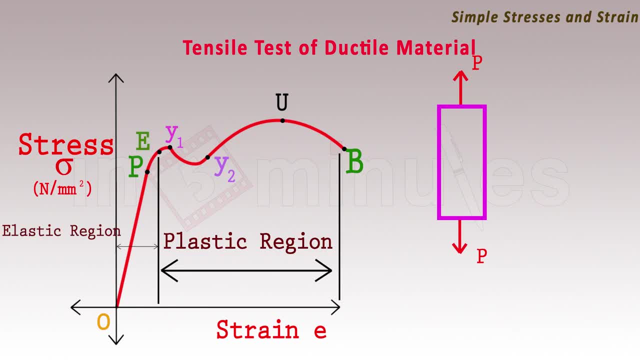 So we see that up to point E the stress strain curve is in the elastic region, Whereas beyond point E the stress strain curve is in plastic region, If we consider the ratio of the strain of the plastic region and the strain of the elastic region.